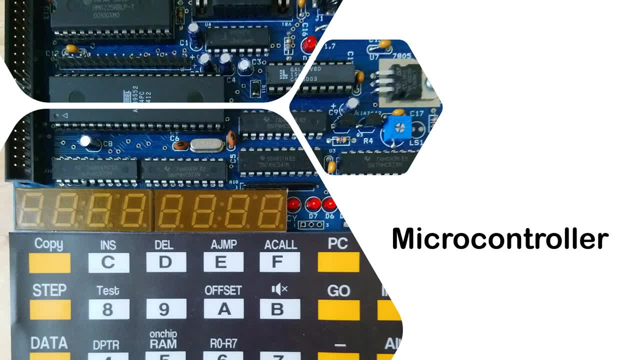 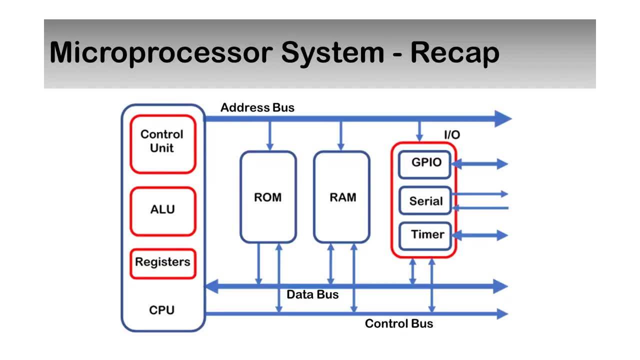 Hi everyone. welcome back to my video series on embedded system. This video is about microcontrollers. In my previous video I explained what a microprocessor and a microprocessor system is. I repeated here the block diagram of a microprocessor system. Basically it consists of a CPU, ROM, RAM. 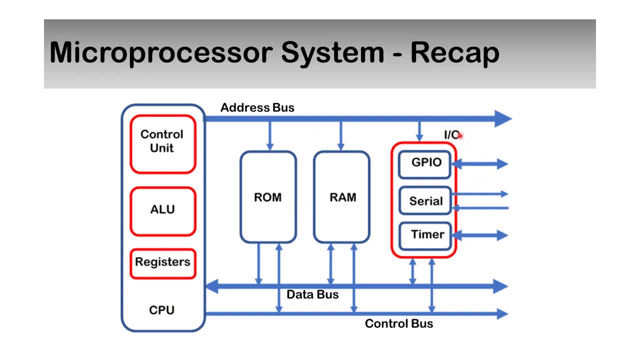 input-output device and all these components- input-output device, RAM, ROM, CPU- they're all interconnected by three buses. One is the address bus. That's the address bus. The other one is the address bus. That's the address bus. 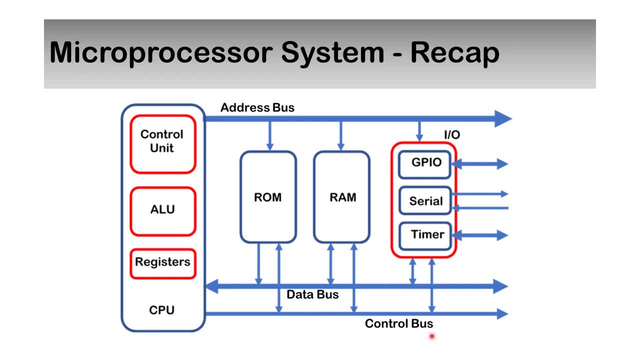 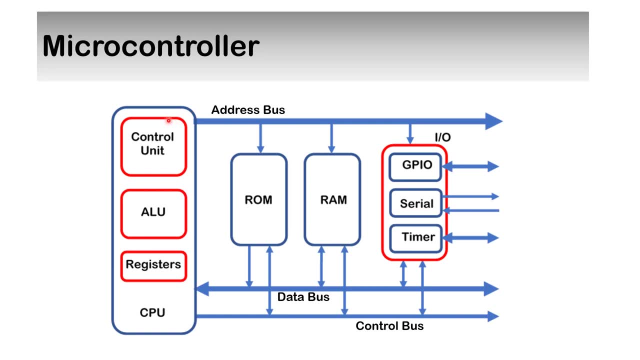 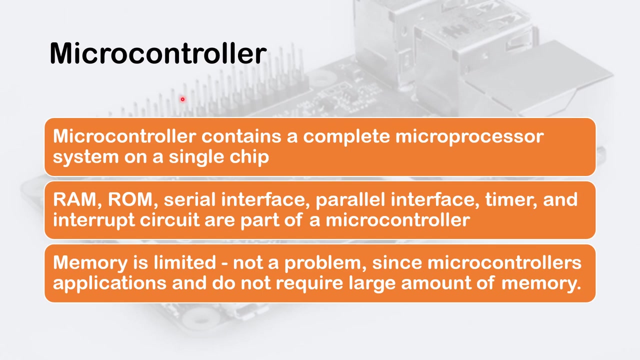 Then there is the data bus and then the control bus. So what is a microcontroller Now? if a microcontroller basically is an entire microprocessor system contained in one single chip, and that's it, That's your microcontroller. So let me just summarize: So a microcontroller contains a complete 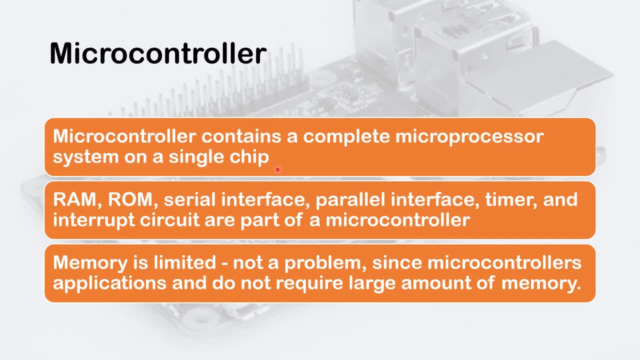 microprocessor system on a single chip. The RAM, the ROM, serial interface, parallel circuit, timer and interrupt circuits are part of a microcontroller. Now, however, the memory is limited, but that's not a problem, since microcontroller applications do not require a large amount of memory. 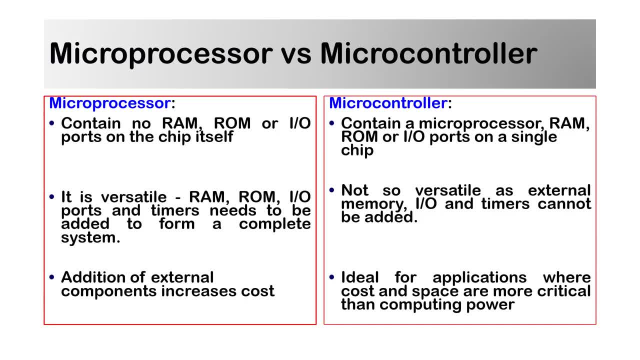 Now, before I go any further, let me just do a brief comparison of the microprocessor and microcontroller. For a microprocessor, there is no RAM, no ROM or input-output ports. on the chip itself, However, on the microcontroller, as we have mentioned earlier, contains the microprocessor. 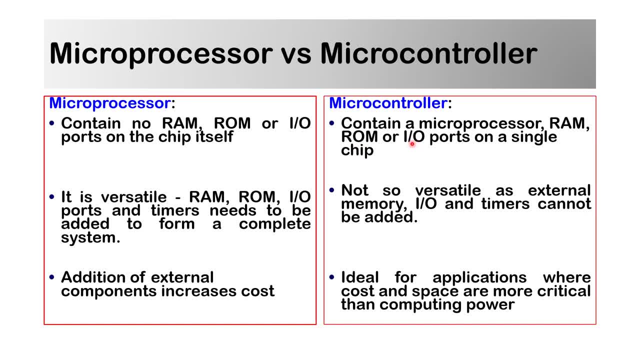 the CPU, RAM, ROM, input-output ports and many more on a single chip. Now, in a microprocessor system it is the microprocessor itself is versatile, meaning you can add RAM, you can add ROM, input-output ports, timers. that needs to be required, sorry, to form a complete system. 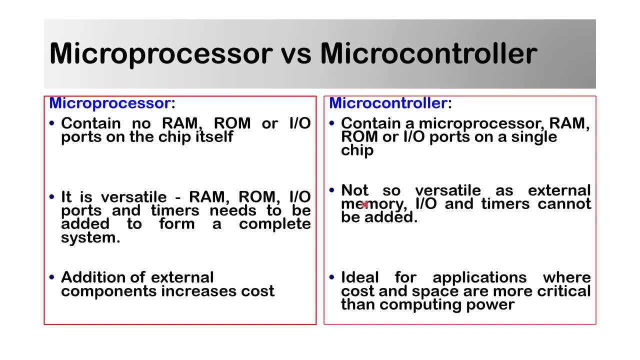 But this is not true for the microcontroller, because the microcontroller itself contains the input-output, the memory, the timers. they're all on a single chip. It's fixed, You can't do anything about it. And one of the other difference is that you need, because you need external devices like ROM, RAM. 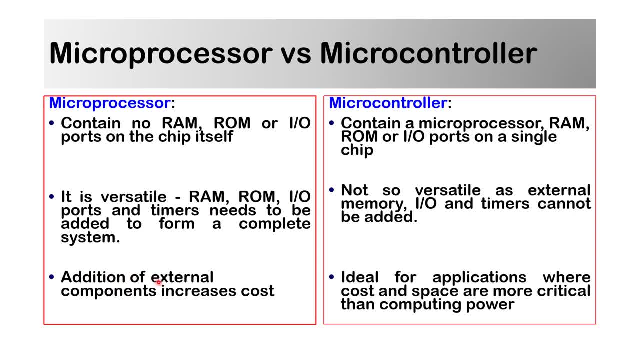 input-output ports. it incurs additional external components, which will increase the cost, But not so with the microcontroller, because it contains the CPU, the IO, everything on one chip. it's ideal for applications where cost and space are more critical than the competing power. 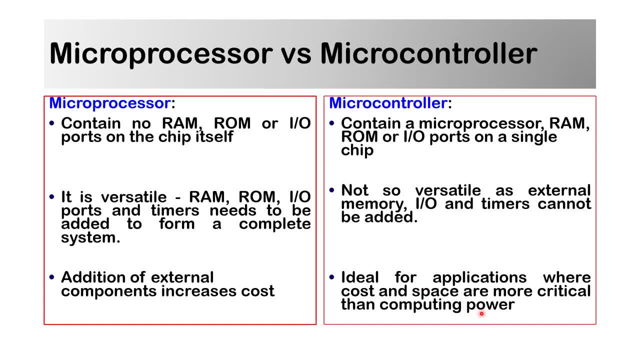 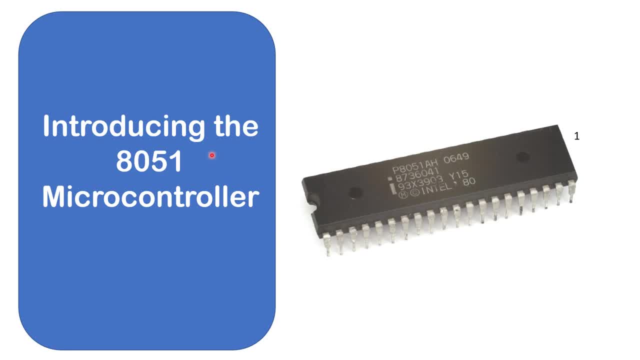 So, basically, this is a very brief comparison of both the devices, And here I'd like to take the opportunity to introduce the 8051 microcontroller. This is the original 8051 microcontroller. Um, let me just give you a brief history of the 8051.. 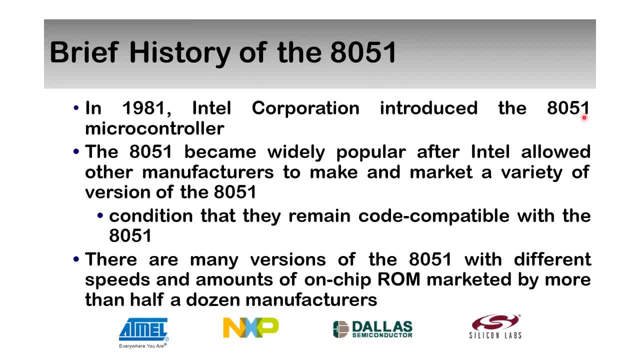 Um. the 8051 was introduced by Intel way back in 1981.. The 8051 since then has become hugely popular. However, Intel do not manufacture the 8051 anymore, but they allow other manufacturers to make and market a variety version of the 8051. 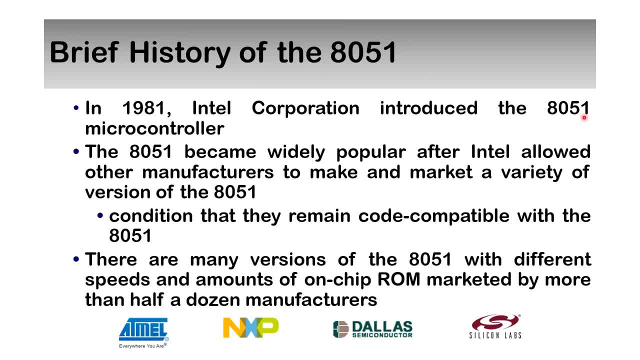 However, there's one condition: that these manufacturers they remain code compatible with the original 8051, the. among the manufacturers there are still making the 8051 are Edmel, NXP, Dallas Semiconductor, Silicon Labs and many more like Infineon and I think. 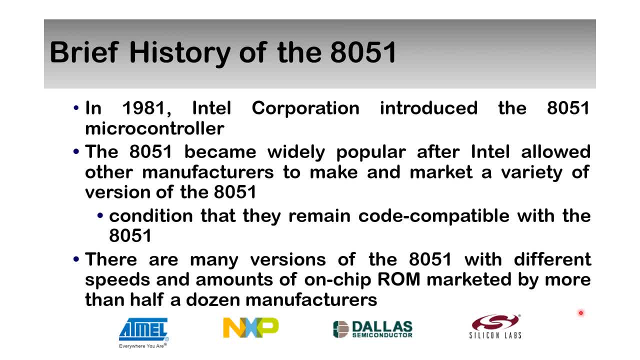 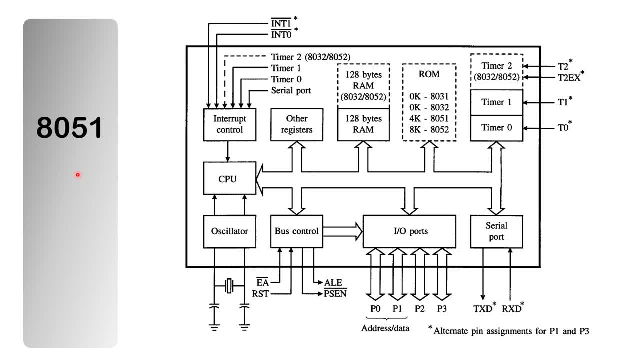 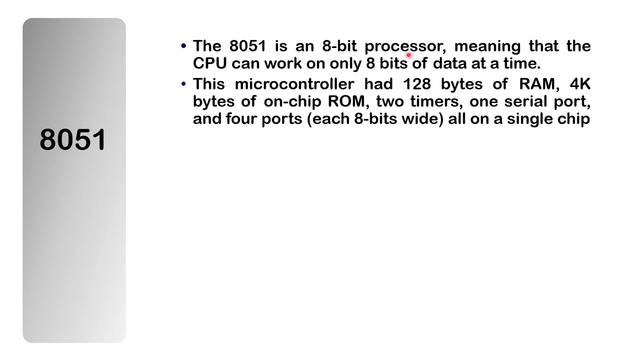 Samsung do make a version of the 8051 now. this is a block diagram on of the original 8051. you have a CPU, the RAM, the ROM, timers, input output ports. there are four input output ports here: serial port and interrupt control circuits. the 8051 is an 8-bit processor, meaning the CPU can only work with 8. 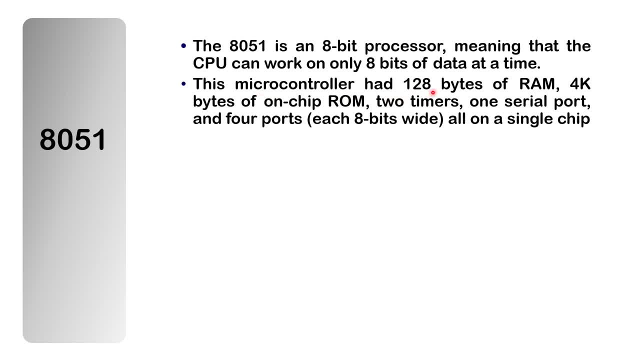 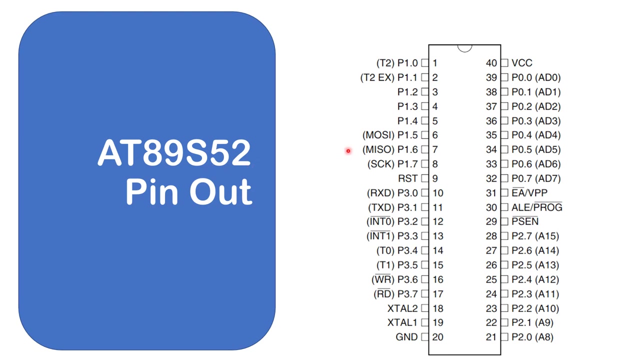 bits of data at a time. it has 128 bytes of RAM, 4k bytes of on-chip ROM, two timers, one serial port, four input output ports, each 8 bits wide, on a single chip, on a single chip. now, this is a pinout diagram of the 8089S 52. I'll be using this 8080 in. 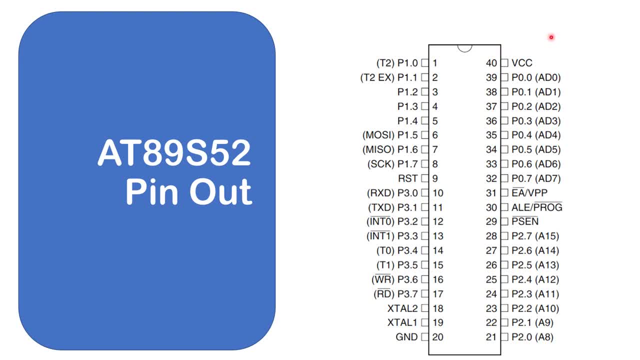 my future video series. here we can see that it contains part 0, part 1, part 2, part 3, and then you have a reset pin here. you also have connections for a, a crystal oscillator. you have the ground pin on pin 20 and vcc on pin 40.. 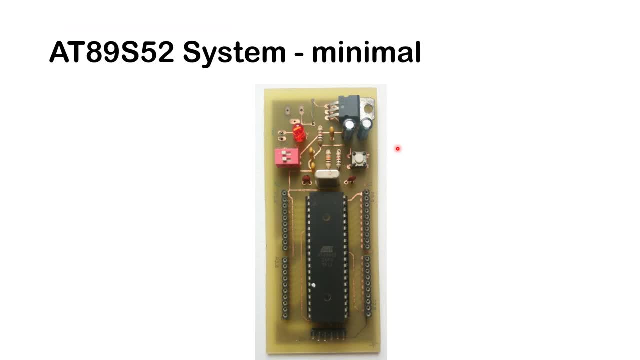 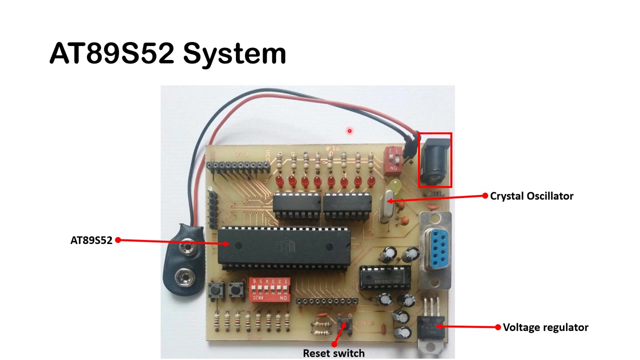 now here's a picture of a AT89S52 minimal system. basically it consists of a AT89S52, a crystal oscillator with a couple of capacitors, uh, the four ports: port zero, port, one port two, port three, a reset switch and a voltage regulator. now what i've done here is i've expanded the minimal system to include on this system here.